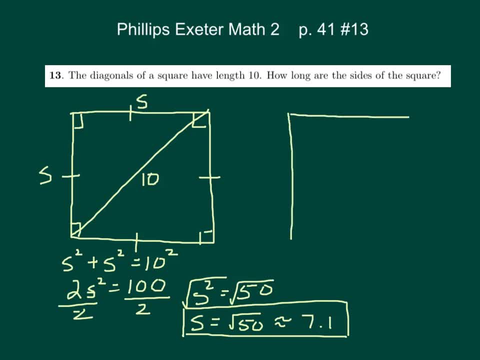 This is not as good, but it says the diagonals of a square have length 10.. So we could draw a square with length 10.. So we could draw a square with length 10.. We could draw a square with both diagonals. 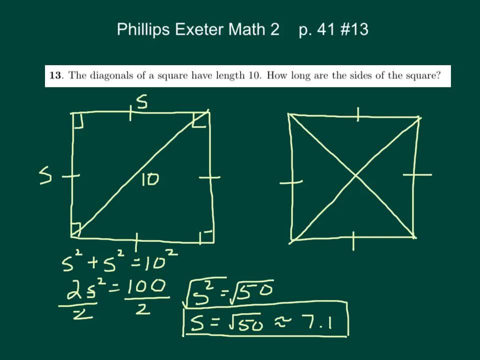 We could draw a square with both diagonals. Both have length 10.. One thing we do know is that, since this is a, This is a square is also a rhombus. A square is also a rhombus. That means that this angle in the middle is a 90° angle. 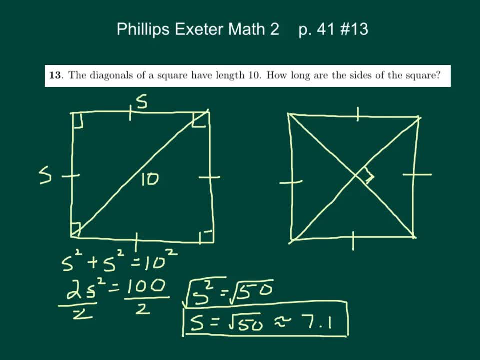 And since they both have length 10, that means each one of these diagonals has to bisect each other because of the parallelogram idea and they're equal. so now we could do the same idea but use this triangle inside and do 5 squared plus 5 squared. 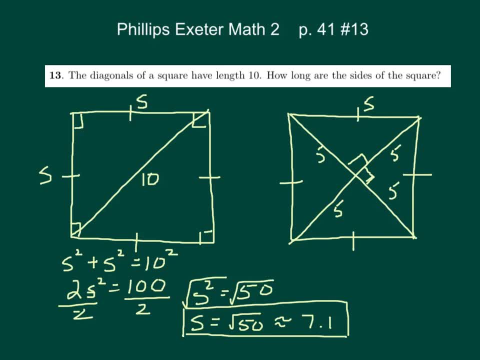 equals s squared. So we could do another Pythagorean theorem there: 5 squared plus 5 squared equals s squared. We work that out, we still get s squared equals 50.. Again, another way we could look at it is if I go back to my original square here. 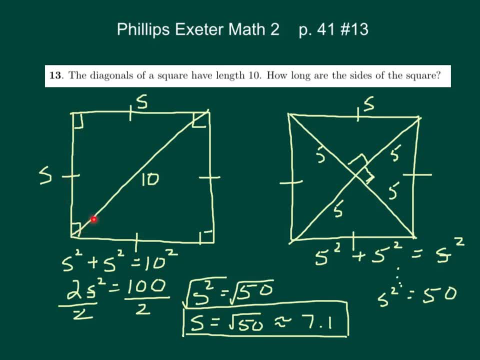 I see this triangle and I know that this triangle it makes is a 45,, 45, 90, because it bisects these angles. And if we remember our shortcut, I'll draw a little one in here with a 45,, 45, 90 right triangle. 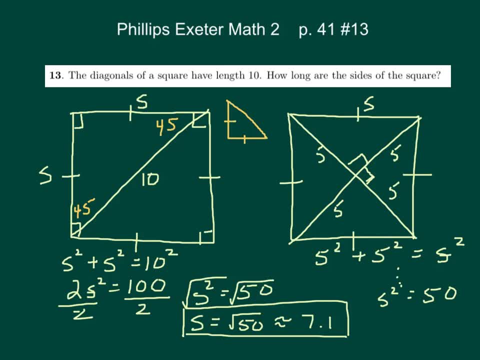 or an isosceles right triangle, which this is. if this is s, this would be s square root. 2: Now, since we're given this side the hypotenuse alongside, and trying to go to the short side, we actually would divide by root. 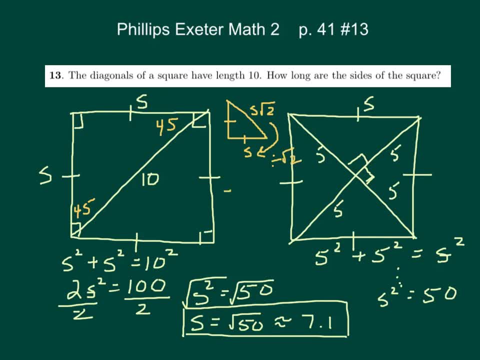 2. So we also do 10 divided by square root 2, which is approximately 7.1. Same idea, Three different ways, same problem.